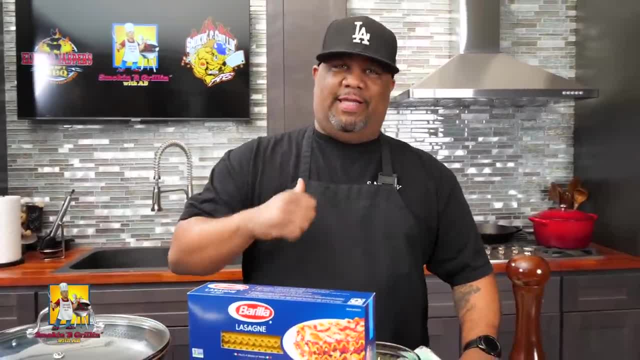 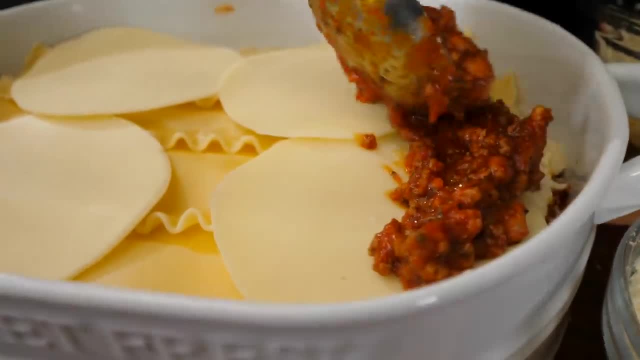 What's good, everybody, and welcome back to my channel, Smoking and Grilling with Me, AB. Now, I know you done seen that thumbnail and you done read that title. Listen, if you've been following me for a minute, you know I do everything on the meaty side. Listen, today I'm gonna show you. 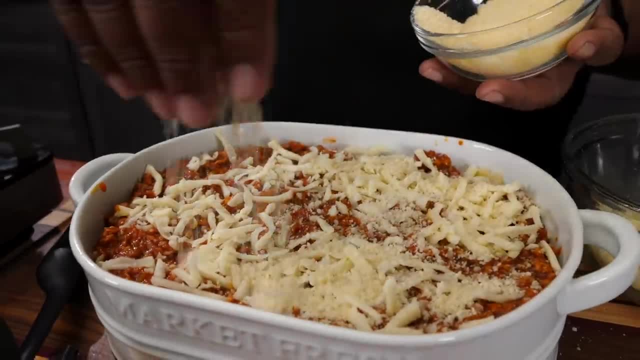 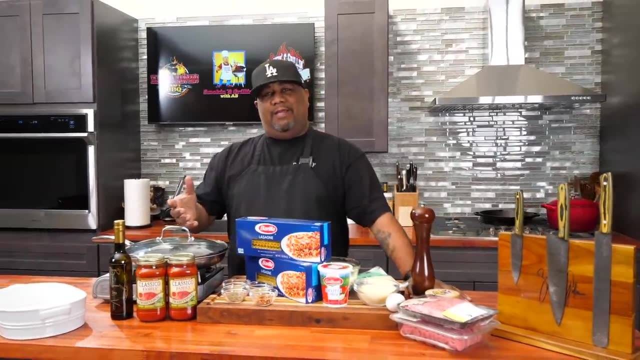 guys just how easy it is to make a meaty. you know lasagna- Super easy. and I want you guys to think about this. Let's just think about lasagna, right, When I think about lasagna, I think about spaghetti, but with a different, you know noodle. and check it out, it got that cheese, Hey, with that being said, 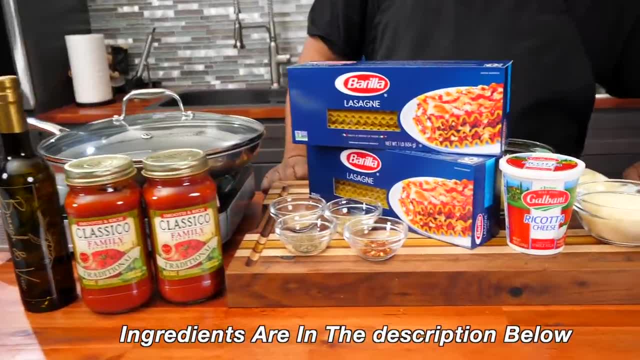 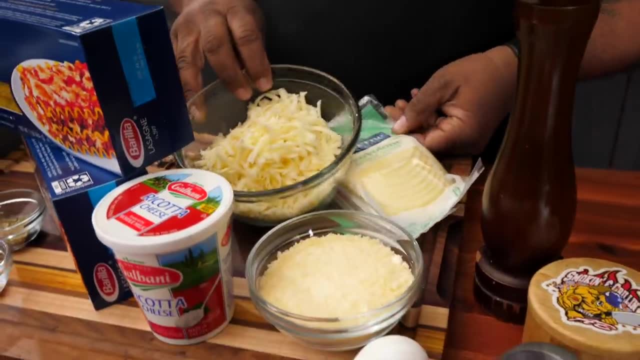 come on in here and take a look at these ingredients right here. As you can see, it's not a whole lot, but look, this might be a little different. I'm gonna be using some of these provolone, you know, slices for some of the cheese. I got fresh grated cheese, more cheese, salt pepper. Look, we got pork. 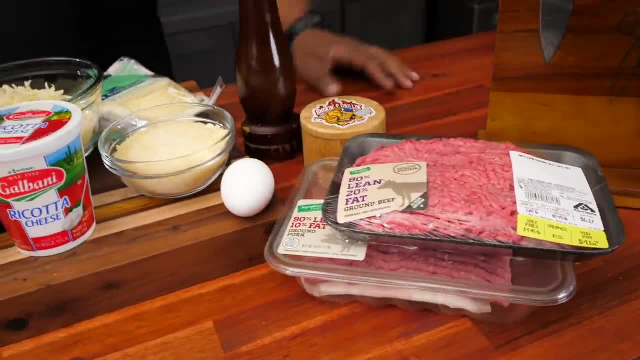 and then we got ground beef right. This says 80-20.. You guys can make it out of 90-10. that's cool. I like to use it on a leaner side, but you know what? I always keep this and I didn't think about having 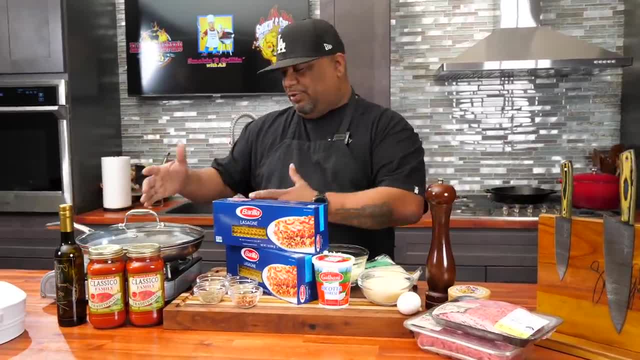 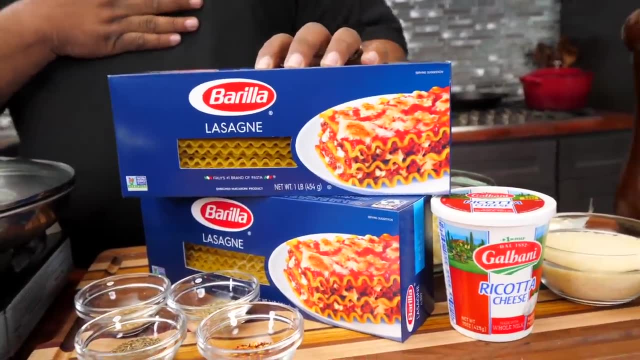 no, lean. you know super lean meat. So if I got any extra grease or whatever, we're gonna strain that. Let's talk about these lasagna noodles Now listen when I make it. I'm not gonna lie to you guys. and look, I want you guys to take a look at the end of this video, Look at the iCard and I put it at the 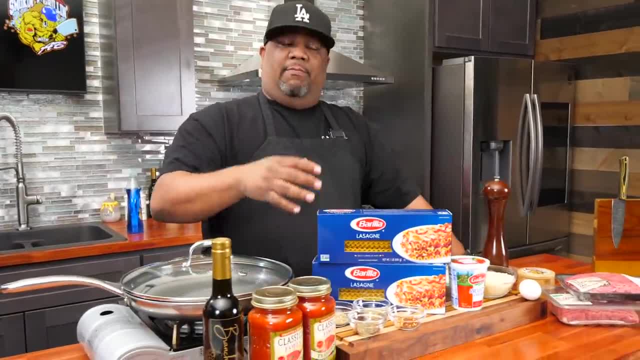 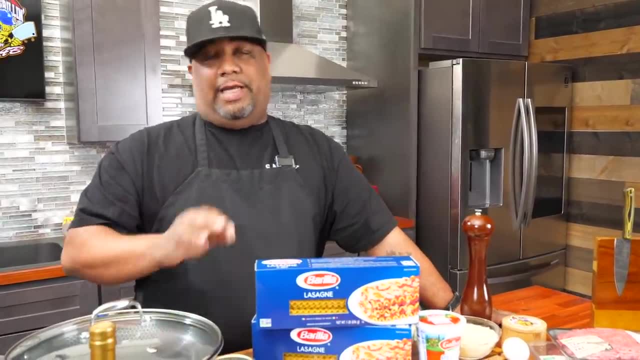 end right, These are. you have to, you know, cook these, these noodles, right. But for me, what I like to do is I like to no cook kind. You put them down, you let everything cook. You know why? because this channel is all about simplifying these recipes and taking the mystery out of cooking. Hey, with. 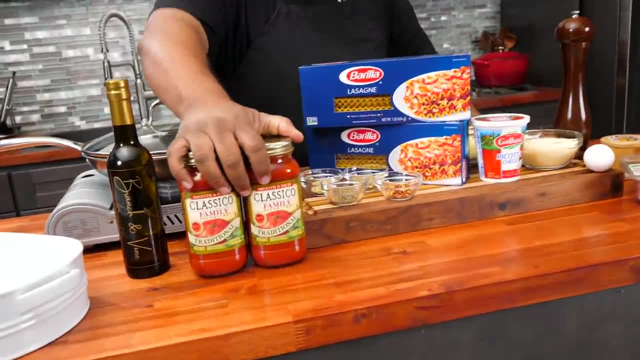 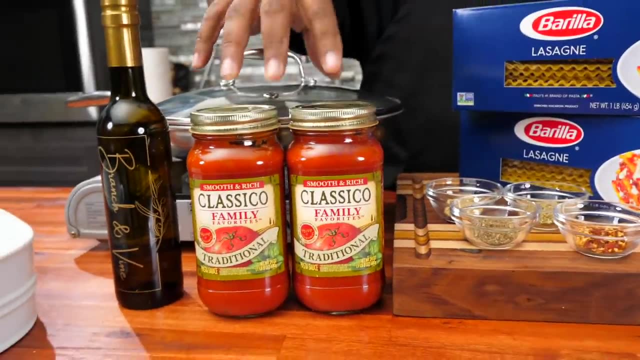 that being said, you've seen all of this right. You can use marinara spaghetti sauce, whatever you would like to do. It's really these ingredients right here. that's what's going to like, just like: raise this up and get that flavor you want. And I want to say this: I always anything. 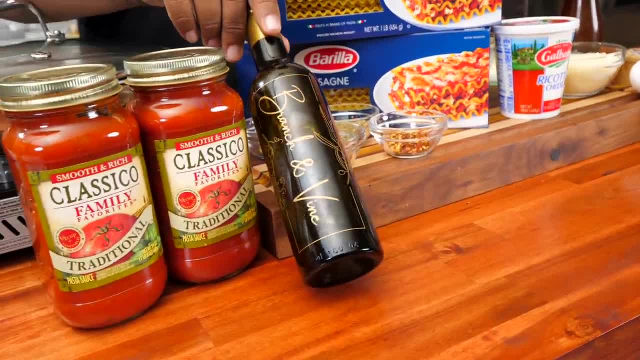 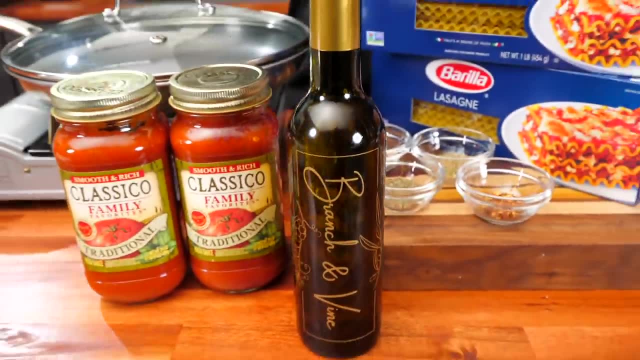 Italian. I'm gonna be honest with you. anytime I gotta use olive oil. this is what I use. you guys, I use branch of vine look infused garlic olive oil. This right here, this is fire. You guys got to have some of this in here. We got several different bottles you can use. You could use. 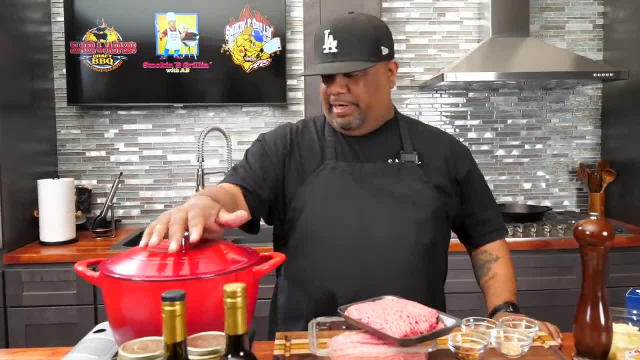 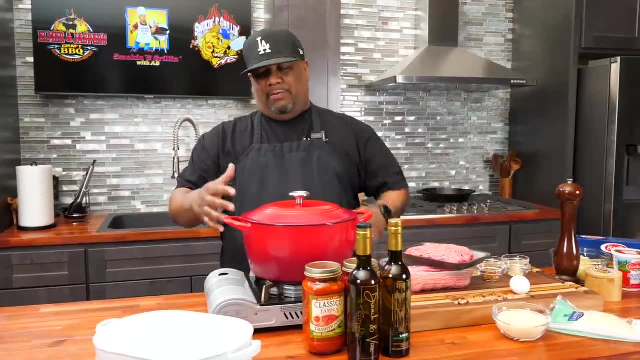 garlic, basil, whatever. We're gonna go ahead and get everything started. I'm gonna use my Dutch oven. We're gonna have a lot of, you know, of our sauce in here. I don't want to like come over the top or have to like stir it gingerly, right, So I'm gonna go ahead and put some set this on medium high heat. 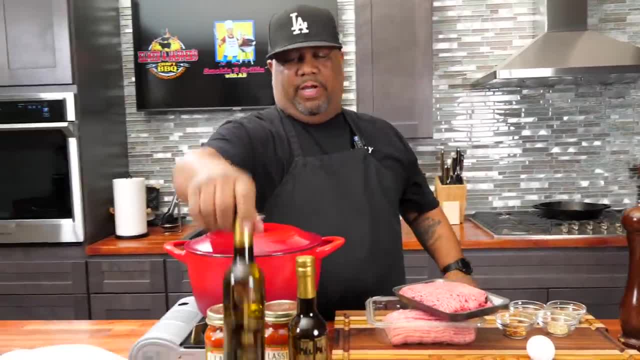 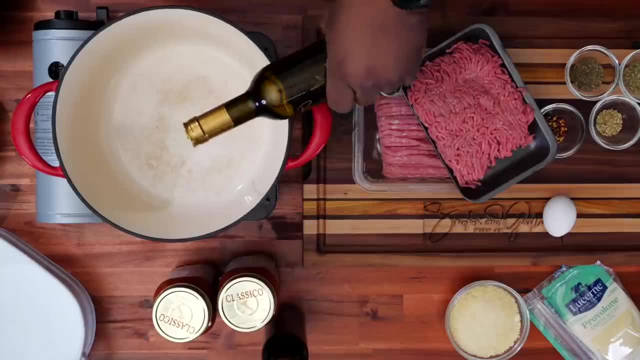 right, We're gonna let this build up a little heat and then, as always, like I told you guys, this branch and vine, these, these infused olive oils. I love them, So I'm gonna go ahead and just put a couple tablespoons in here right now. Listen, I understand that we're using pork and ground beef. 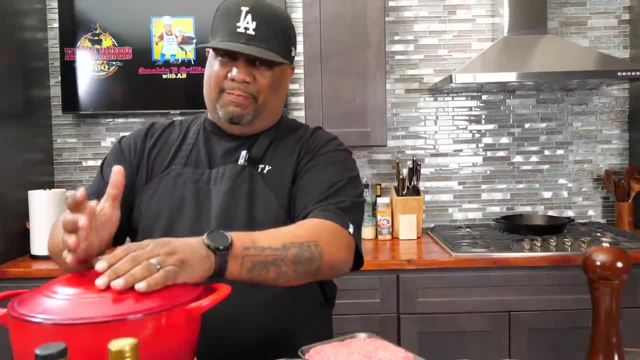 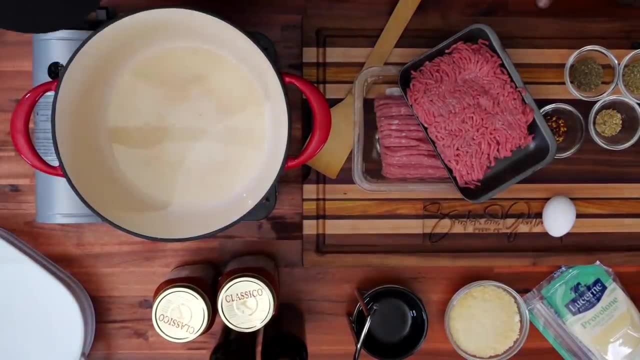 and all that stuff, but it's gonna make the sauce a little more�ucous and it's gonna just render down this own fat also. but listen, we want to give it a nice base. We're gonna start with that right there. we're gonna infuse it with that and this, okay, So look, oh my goodness, that right there is. 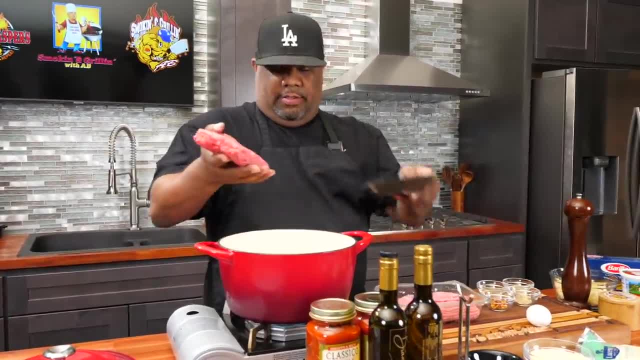 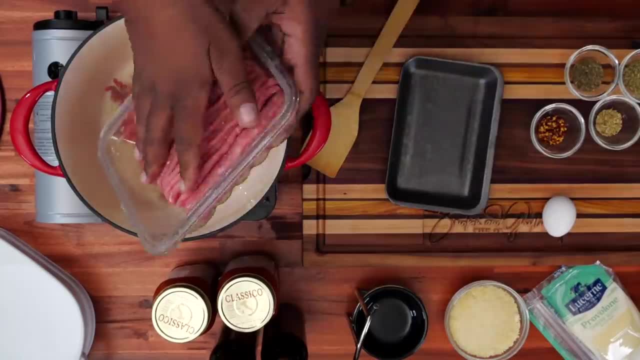 fire folks Just to smell that infused olive oil. that's the way to go. Now I'm gonna go ahead and just add it. now, look, I want to add it away. Don't just drop it in here. as you can see, it's nice and hot. 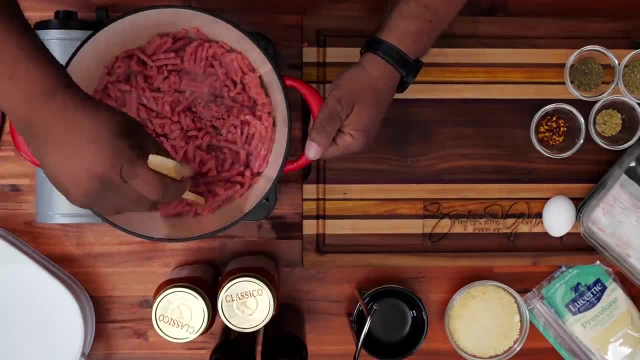 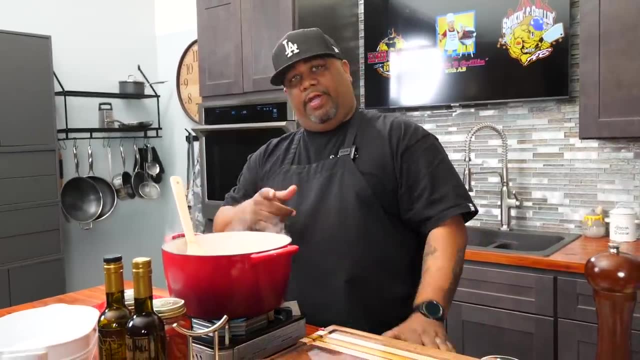 Now, what you see me doing is I'm just breaking it up. I just want to get you know maximum coverage on the ground, on the bottom, and I'm gonna let this cook folks, Once this cooks, then we'll start flipping it over and breaking it down. Okay, so look, now would be a good time for you guys to cook your, your pasta down, right. 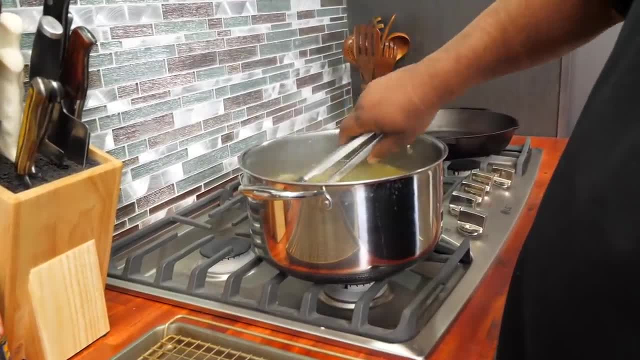 I'm gonna get these tongs and I just want to handle them, coat you know, and make sure I'm careful with them, right Eight minutes. We just want them to be al dente. I use a baking sheet and we just lay them right here. 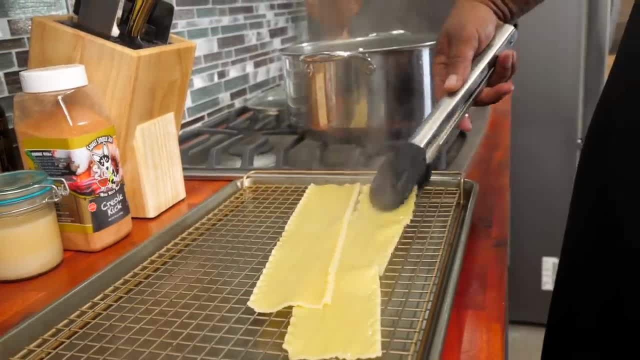 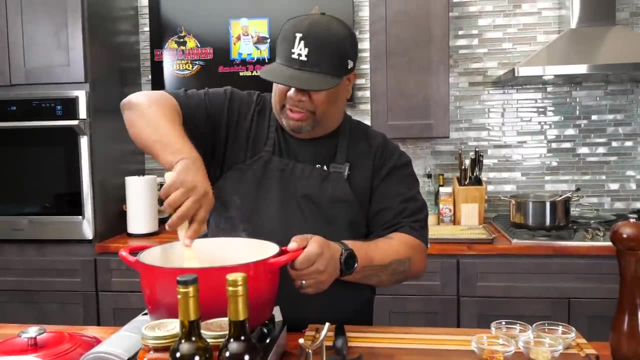 right, We'll just do just like that. now I'm not gonna bore you guys, I'm gonna just tell you you want to do this and you just want to dry out, you know, Okay? so look, as it's starting to cook. Obviously it's gonna turn brown, right. 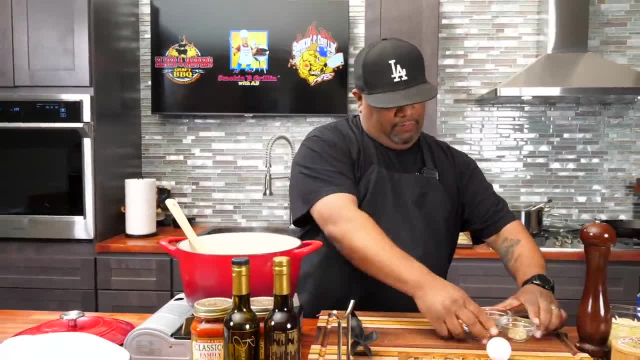 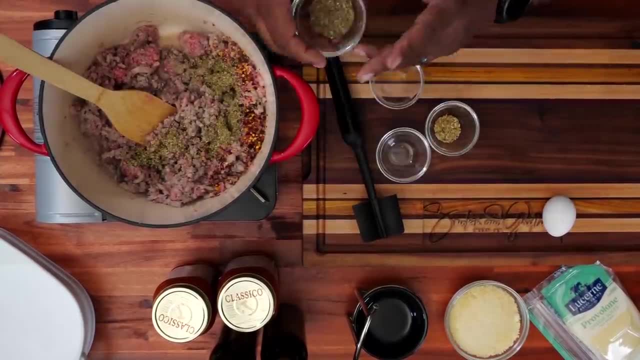 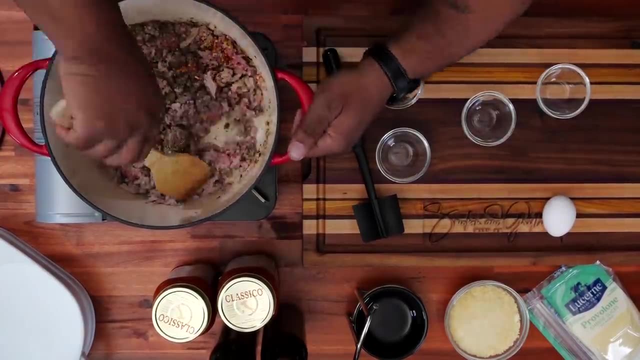 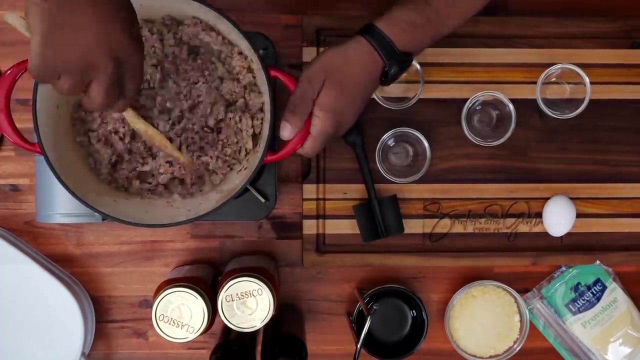 So, look, I'm just doing a little break up here. Now. You remember all of our dry seasonings. check it out. We're just gonna sprinkle it In here, just like this Right, and now we just gonna mix This right. here is gonna be some flavorful and meaty, you know, lasagna. 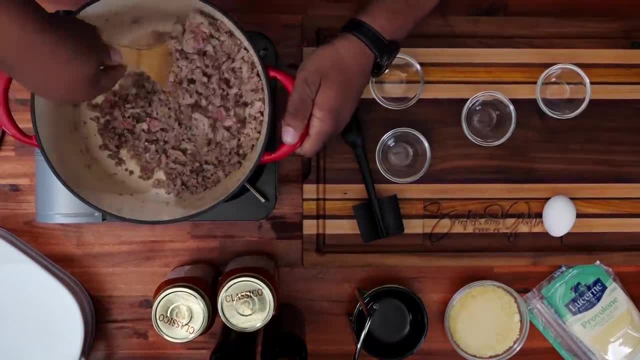 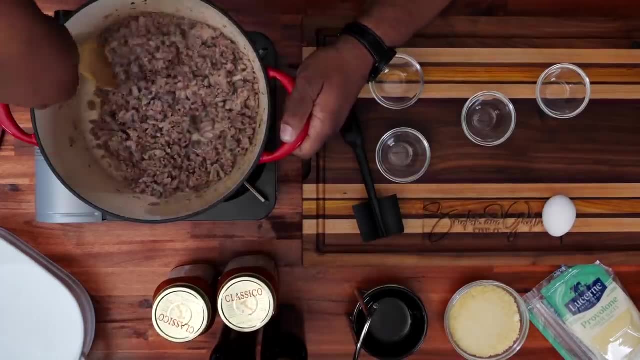 Now, for those of you guys that don't do the pork, I obviously you could have just did two pounds of you know just a you know ground beef. And for those of you guys that want to do something different, What about? don't forget about it, Listen, I don't have chicken lasagna, turkey lasagna, I'm gonna let it. 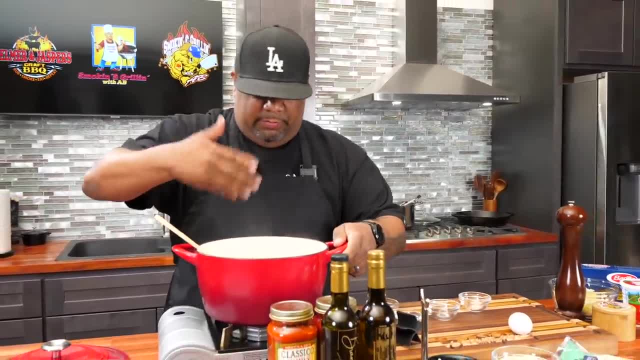 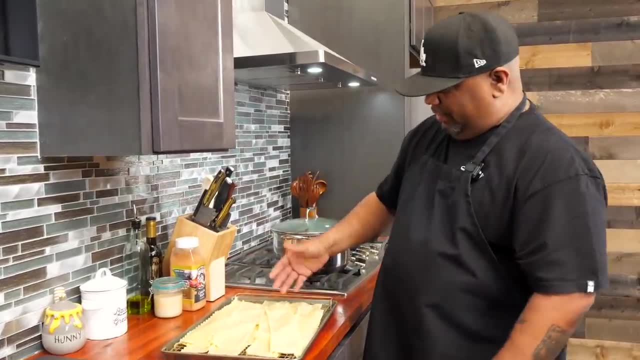 Continue to cook. We got it. Oh, oh man, just That right there. This is how you know it's gonna be fireproof Folks, okay, So you can see. I just lay them out like this. look, they already cook and I'll you know. 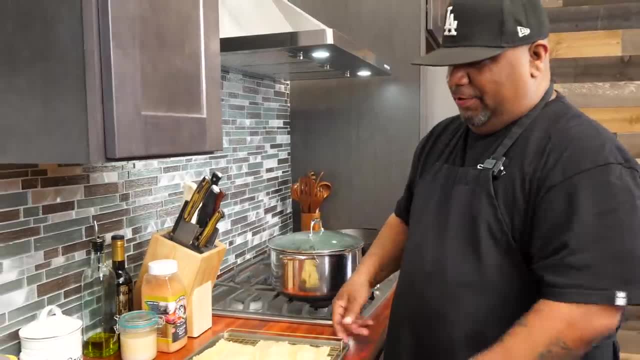 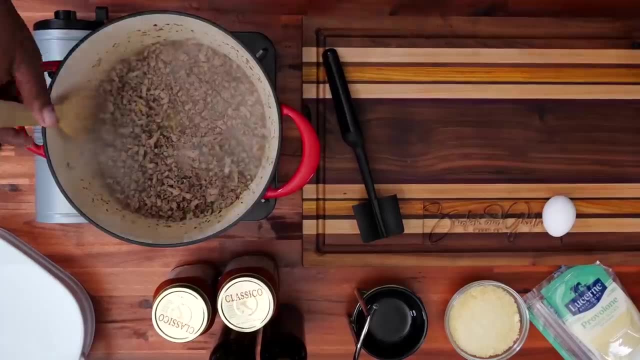 So they can like halfway, you know, dry out, and these are already ready Cuz. look, the rest of it's gonna go fast. if you guys didn't know, lasagna is so easy. It's almost. to me It's like just making a hamburger, Okay. so you see how that's cooking down. you can see it render. 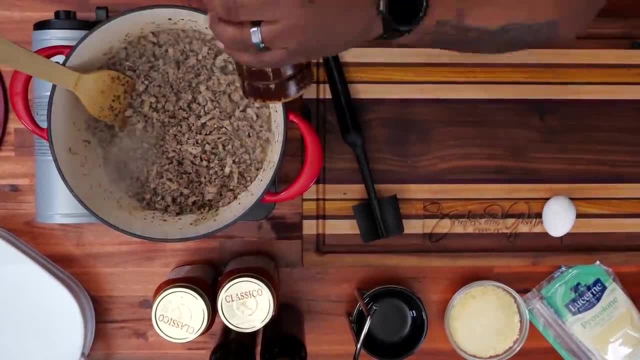 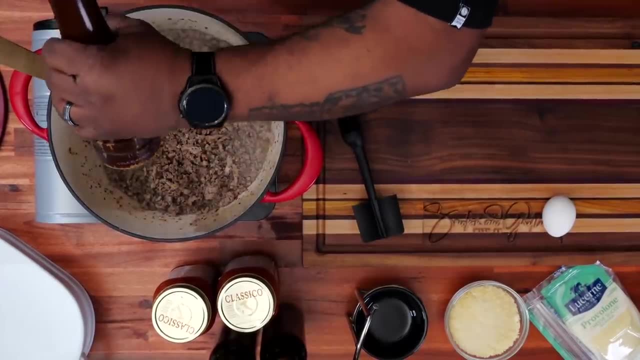 But we gonna get rid of some of that, right? What you want to do is you want to get your salt And you want to get your pepper. Now, if you guys been following me for a minute, you know- I like to tell you you can't put enough pepper. 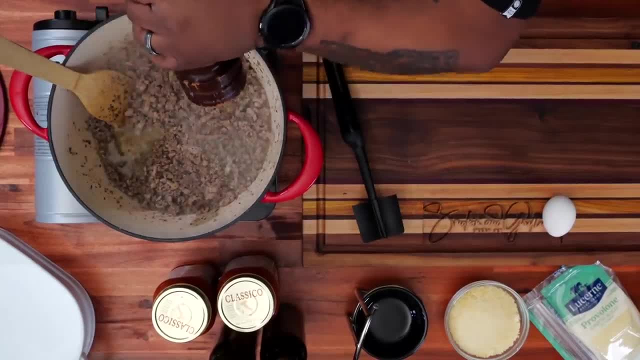 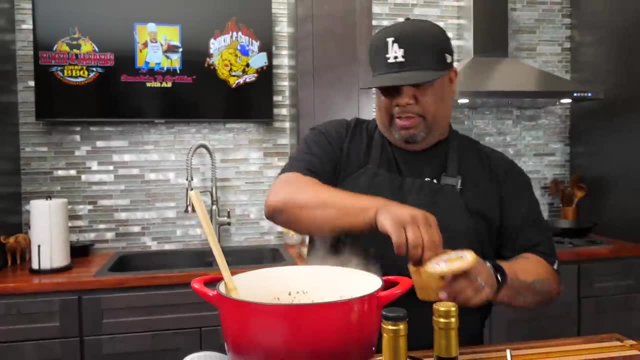 Black pepper in here, So I'm just gonna keep going until my arm gets tired. Hey, just a Roman from all of this coming up. This is perfect right now. a lot of meat, right. So I'm gonna give it a couple of generous pinches of salt, and that will probably do it, if anybody else need any salt. 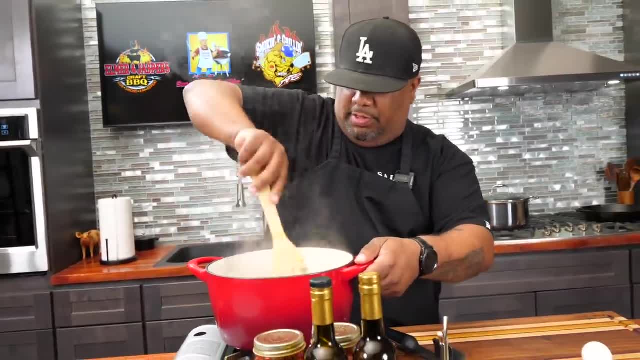 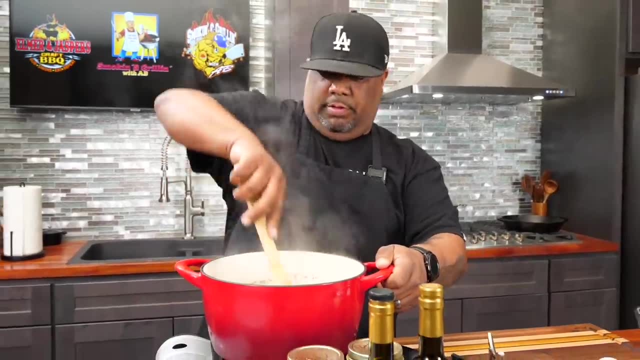 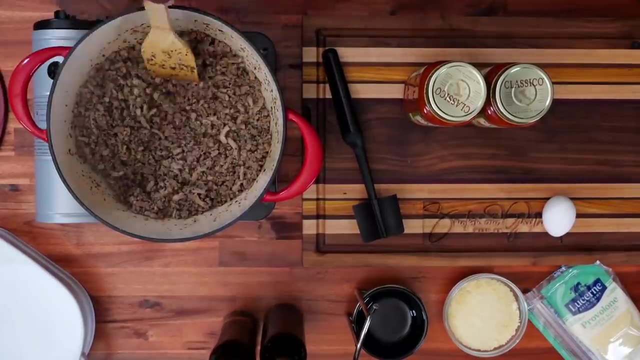 They can, you know, put some on their individual pieces, you know. but that right there, if you watching your salt intake, This is gonna do it. Now I'm gonna turn this down on low And we're gonna move to the next part. Okay, so look, I just drained off the fat, as you guys can see. look at that right there, You can hear it. 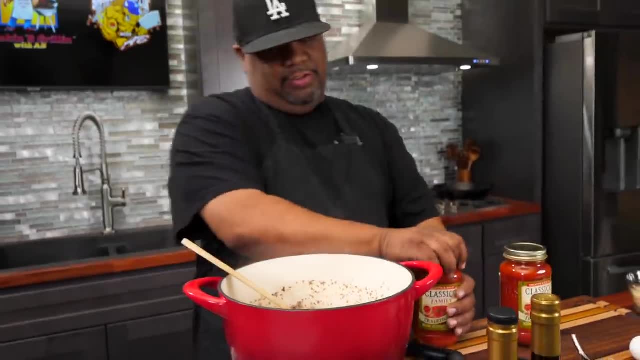 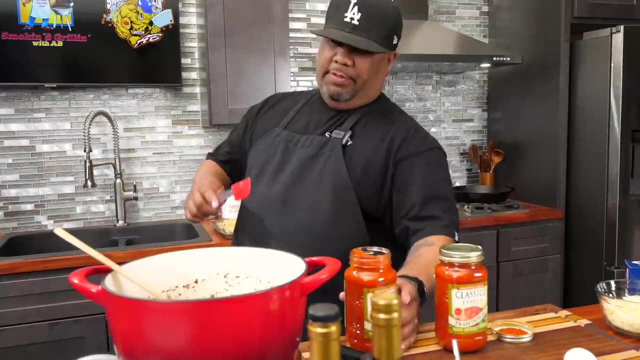 I got heat under here. I went back with that medium-high heat, right. So now it's time for us to add whatever sauce that you guys are using. You know, I mean, we doctor this a really, really nice. We just want to have the right tools for the job. 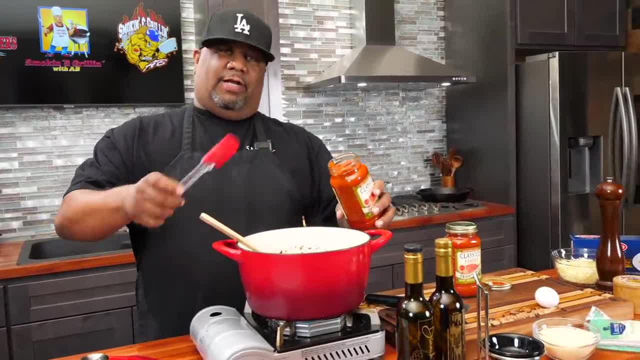 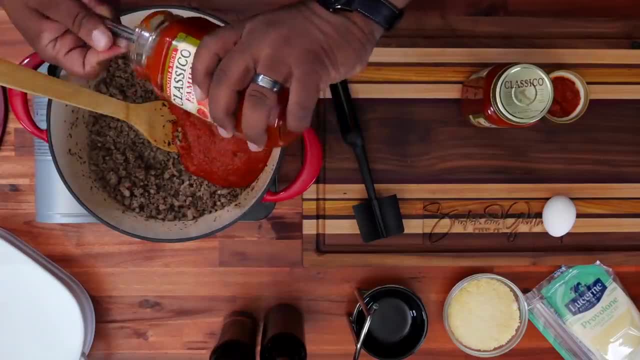 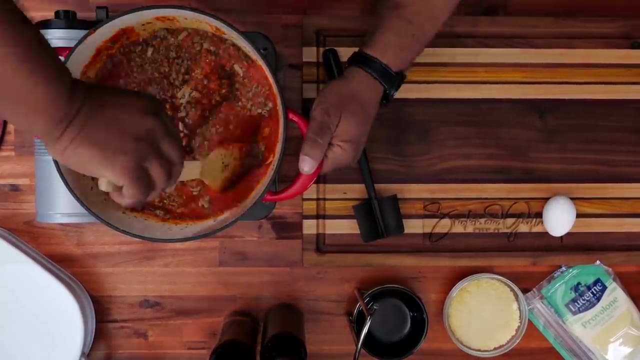 I want to get all of this out. Everybody know, once we get it out, I know a lot of times we put a little water in there, put the cap on, shake it and then pour it in there. right, There we go, Come on. Okay, so got that in here now. What I want to do is just mix it up, right, remember in the beginning. 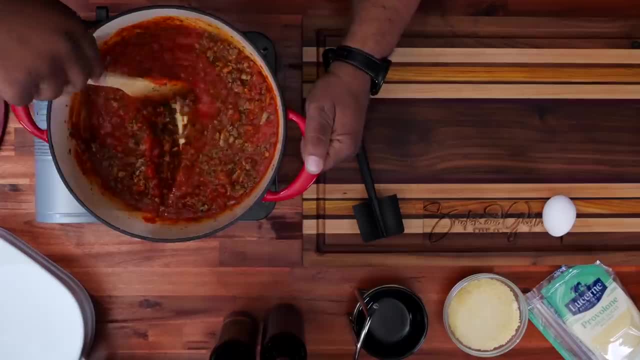 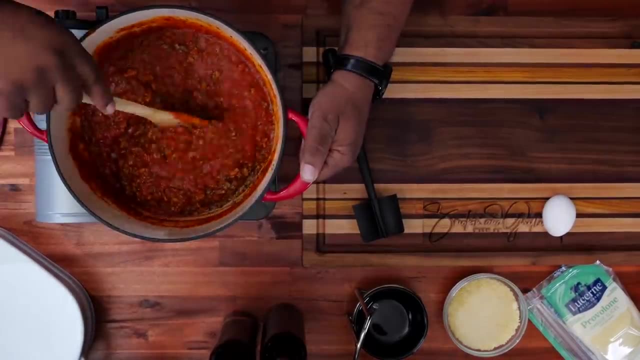 I talked about spaghetti, Right, You see how it's coming in. This is how I like my spaghetti, you know. but I like to make my sauce, You know, from scratch. I made it. I'll put some links in here so you guys can take a look at it. 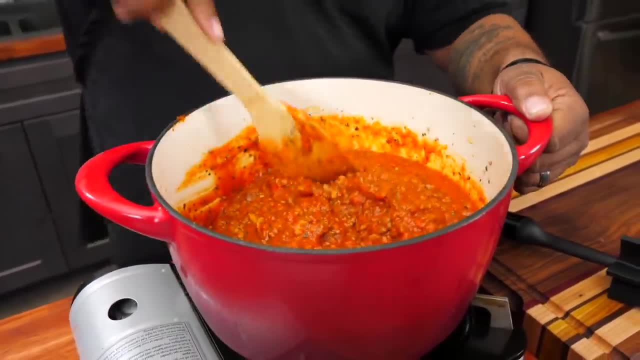 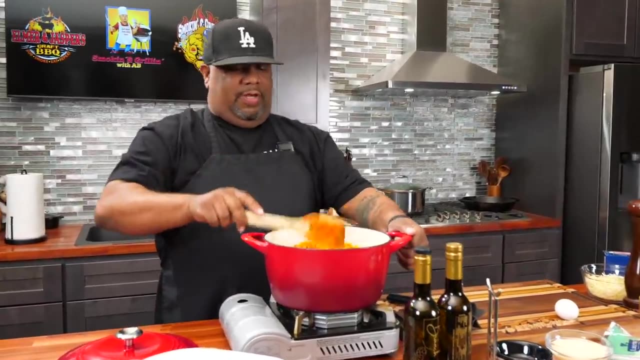 It's up to you. But remember, we just keeping it simple. We're looking for a good meal That's over the top, That's easy to make. Not only easy, but fast, Right So now I want to go ahead and let's just come up to a simmer. 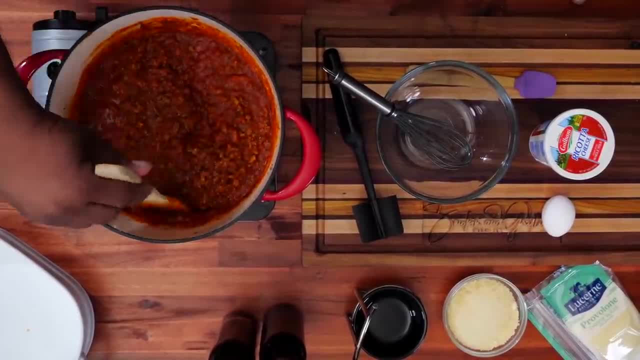 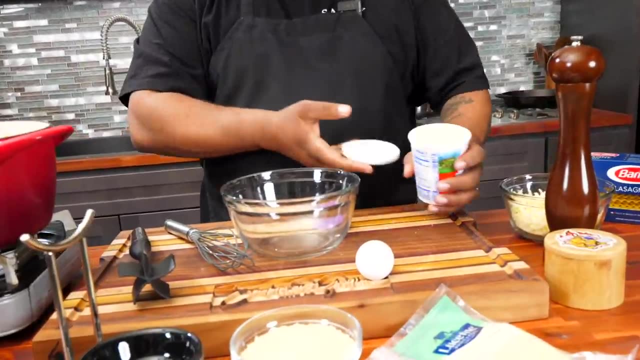 Okay, So while we letting this come up to a simmer, really what it's doing is just heating up, you know, Our sauce and mixing everything together, right? So while that's happening- that's on its way- Let's go ahead and take our ricotta. 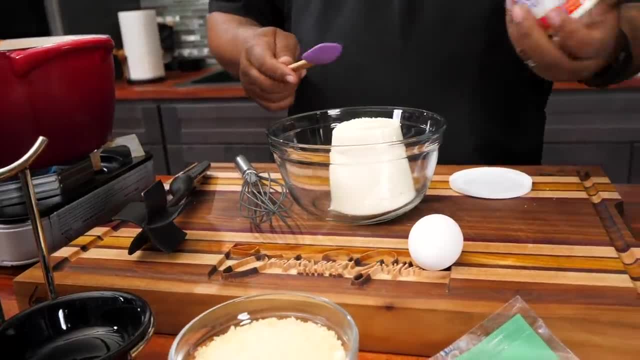 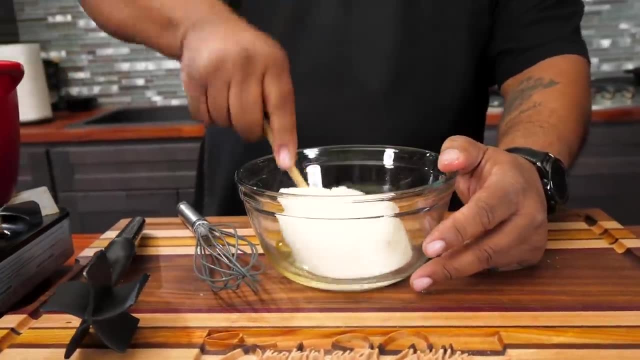 Let's just go ahead and add this, you know, to a bowl. What you want to do is you want to mix this. We're gonna add this egg, Right, I'm just gonna break it up first. Now, I'm just gonna give this a whirl, just like this. 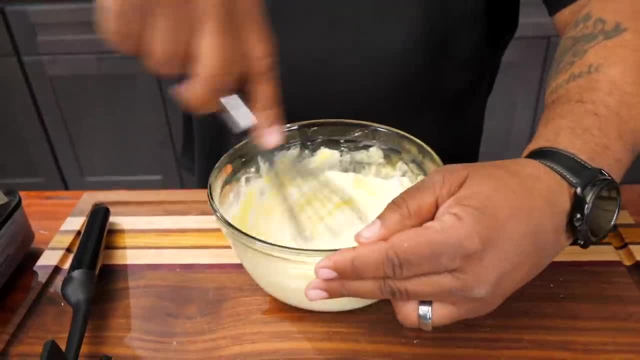 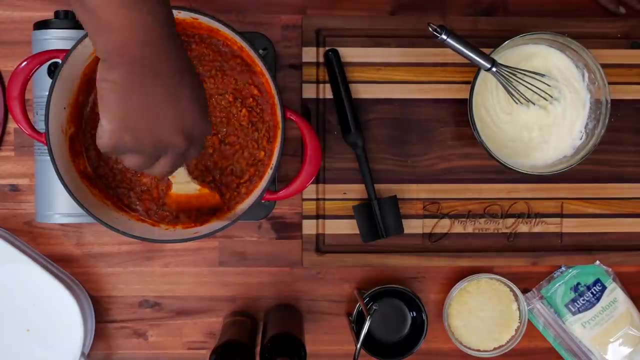 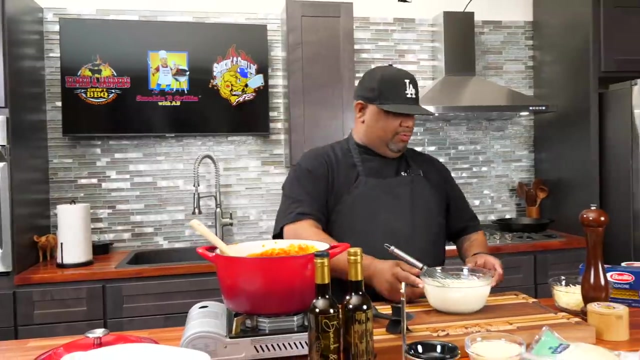 We just want to get it mixed up Now. once you got it all mixed up, like you see right here, look at this, right here, We're already coming up to a simmer, you see that? So look, I'm gonna reduce this down to the light low. We just want to keep it nice and hot now. I guess what, folks? it's assembly time now for the good part. 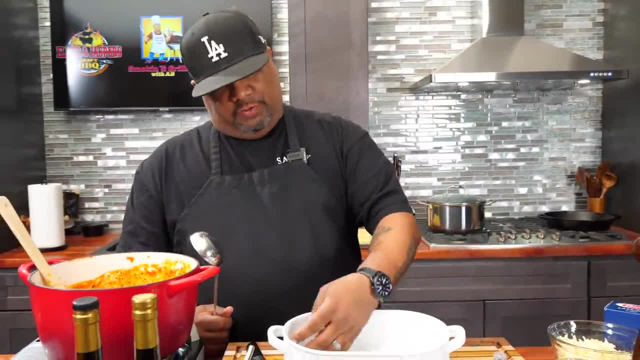 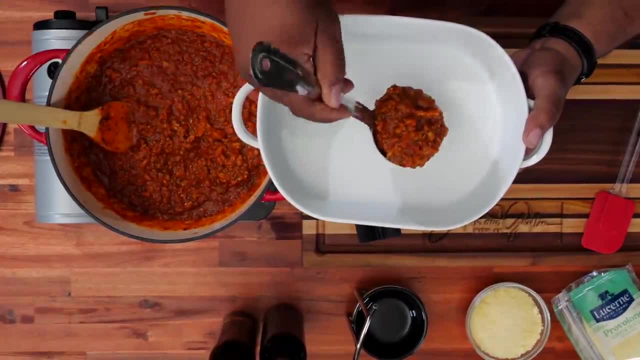 Now we're gonna do the assembly. So listen, I don't need to spray this. why? because I'm gonna take some of this meat sauce and I'm gonna put this down on The bottom right, So we'll just do it like this. So we're just gonna do it like this. 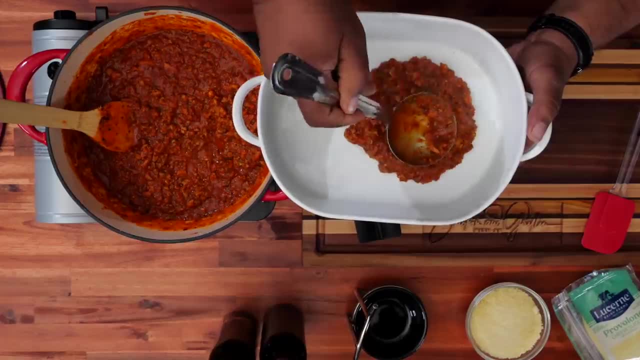 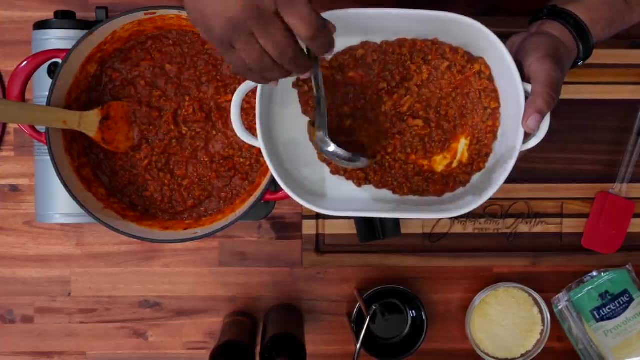 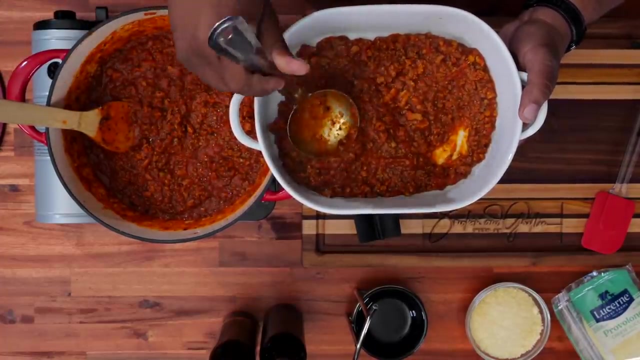 Right, Then we just want to make sure it spreads. you could just use the back of you now. I should have probably said this: look, 13 by 9 works great. I Should have said that from the very, very beginning. Now you guys can see just how immediate this is and you can see that why. this will give you an explanation. 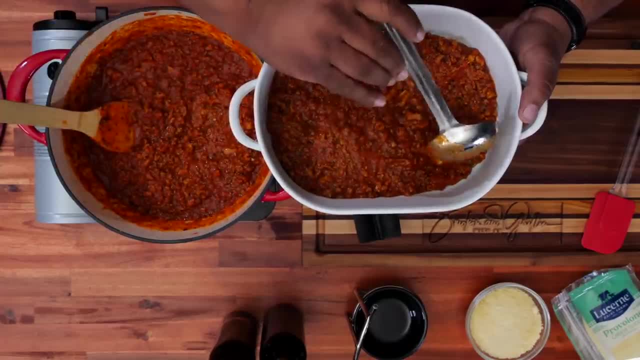 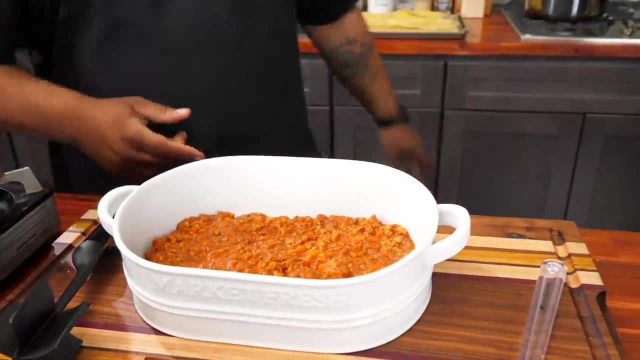 With your eyes why it won't stick right. So we just put a little layer. It's probably like about a quarter of an inch stick and this right here, but a 13 by 9 is what you want. now you see my noodles back here. they already done. i'm gonna go ahead and bring these in. 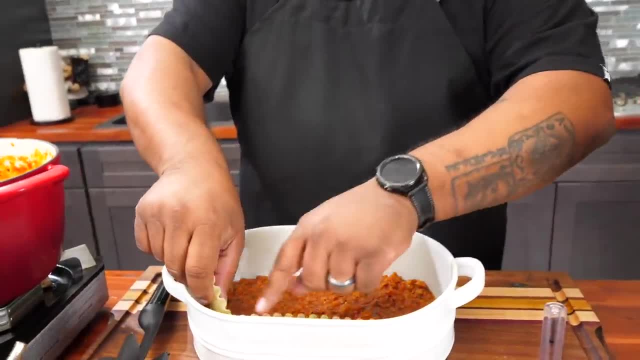 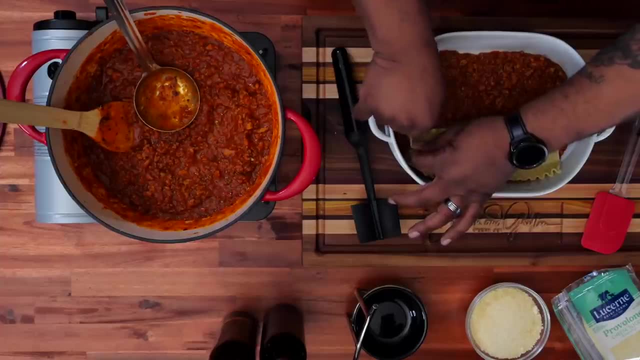 and we just put these in, just like this 13 by 9 square dish, probably be the best. i'm gonna tell you guys why: because then you won't have to do any of this tearing or nothing like this, but for me i have to do that. why? because, for one, i like this little dish that i have, you know. so we'll just 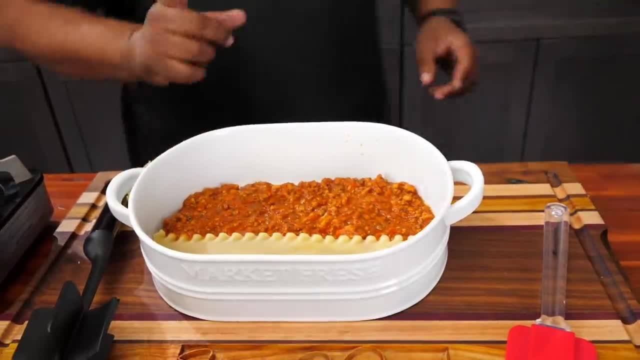 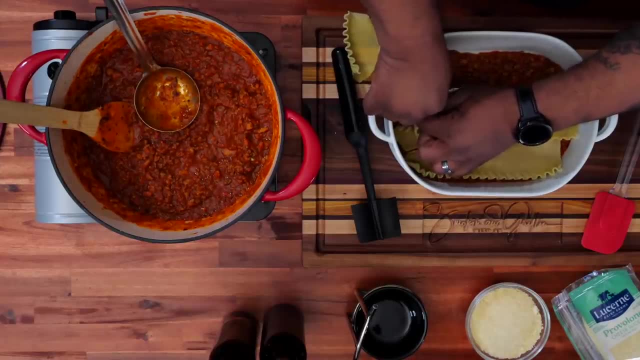 put that in there like that, and then i'll just i'm gonna save this off to the side. i'll show you why. in just one second, you guys can tear it, cut it, use scissors however you want to do it, but if you're using a 13 by 9, like a, like a rectangle dish, everything will just come out pretty much the 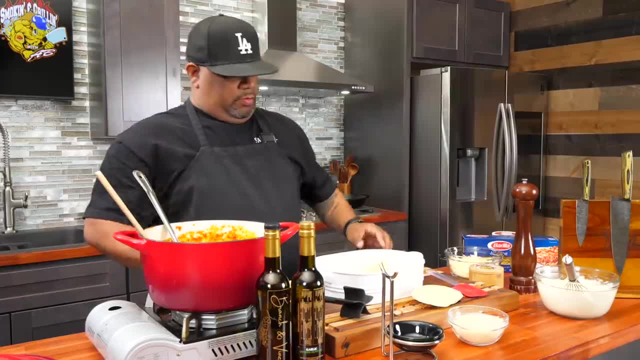 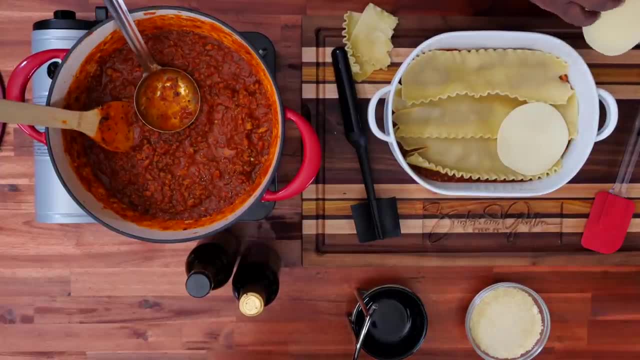 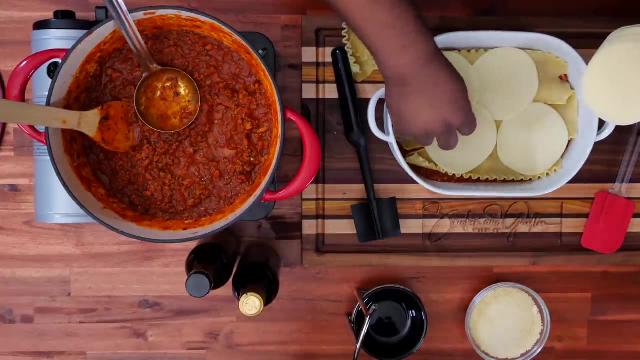 way you want it to be, but this is the way i'm gonna do it just now. okay, so we got that done. now, look, i'm just going to take four slices of this provolone and just add it there, here, here and here. that's good, right there. 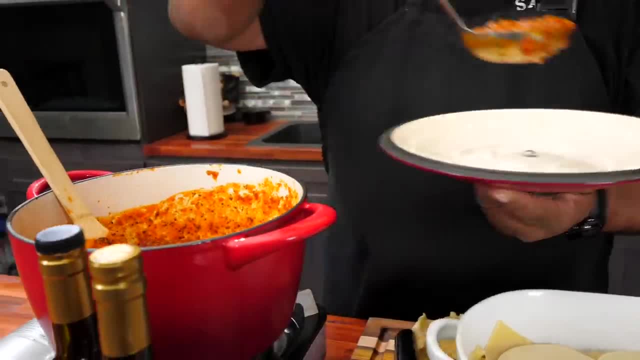 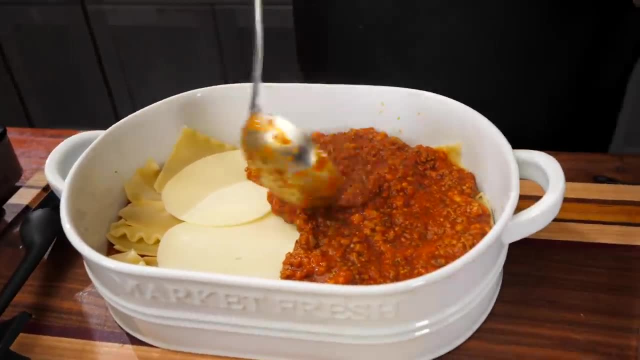 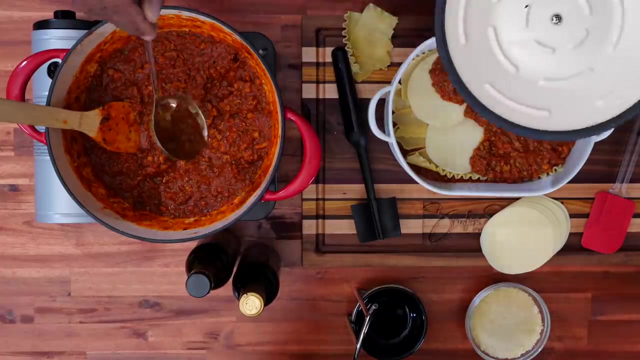 look when this melt that tie them noodles together right now. we'll just come over here like this and then we'll start adding this. so what we're doing is just building layers. you all seen lasagna, so you know how you know it turns out. now you start understanding why we got all the layers right, but we're gonna make this have. 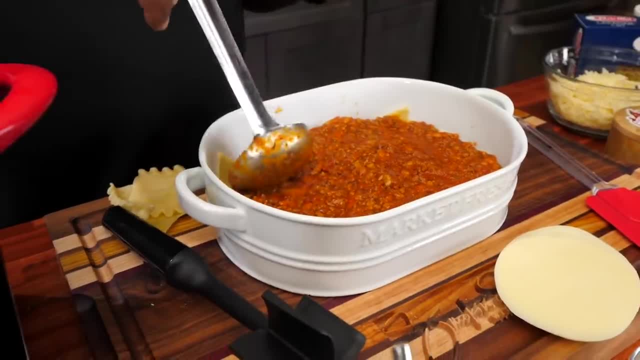 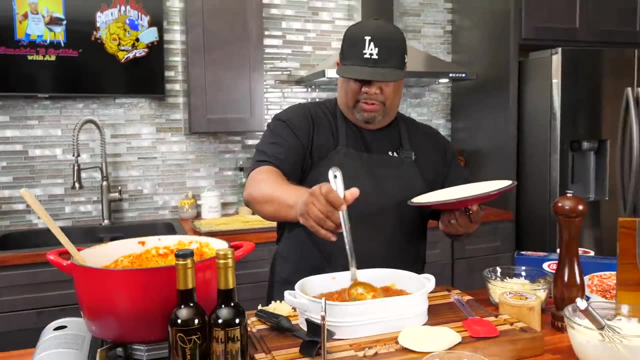 a whole lot of goodness in these layers right here. you guys make sure you don't put too much in there. i guess really, you won't know until after you finally made it. you know, and it depends on the size dish that you're using. but this right here is how i like to see it check this out. we're going to come with that mozzarella. 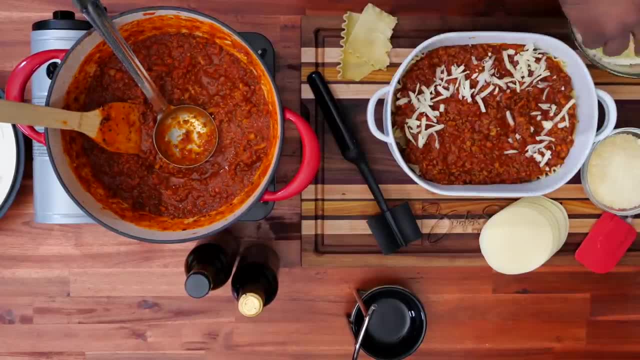 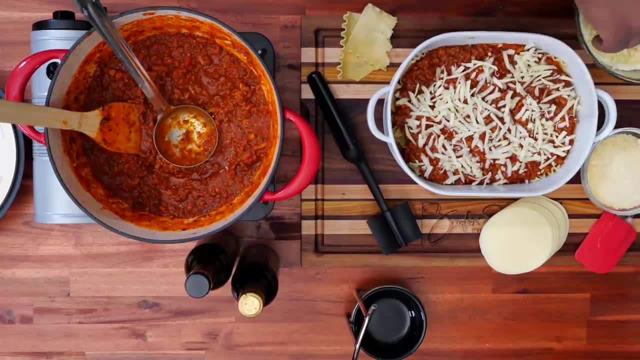 look, don't do like me. anytime i work with cheese, i always end up putting way too much cheese. you know, we just want to use about a quarter of our cheese that we have right. so that right. there is going to be enough of that. now we're going to do the same thing with 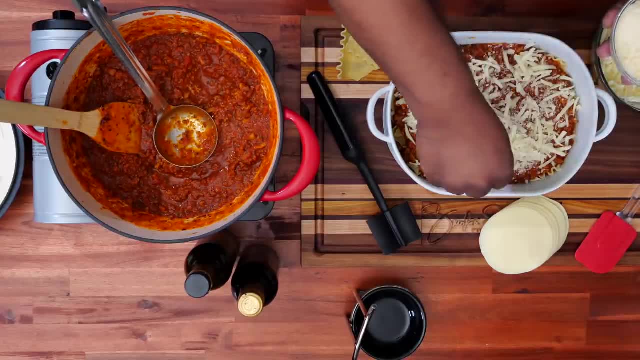 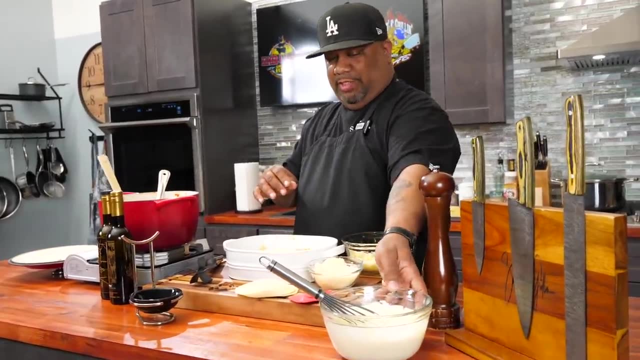 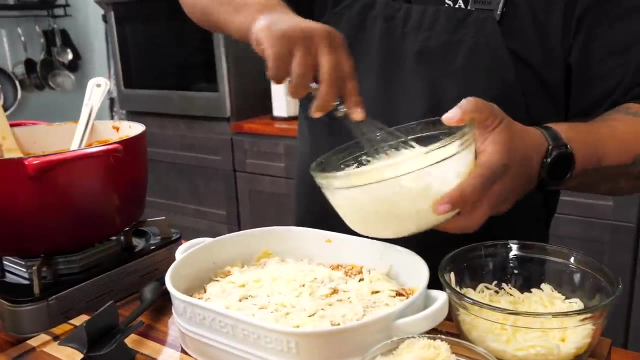 this parm, you know. i mean we just want to kind of like dust it about a quarter. this would be good too. i know some of you guys saying, man, i want mine to be way more cheesier. you guys do your thing. i care more about the meat and the blend, right. so now i'll take my ricotta. just give it another little. 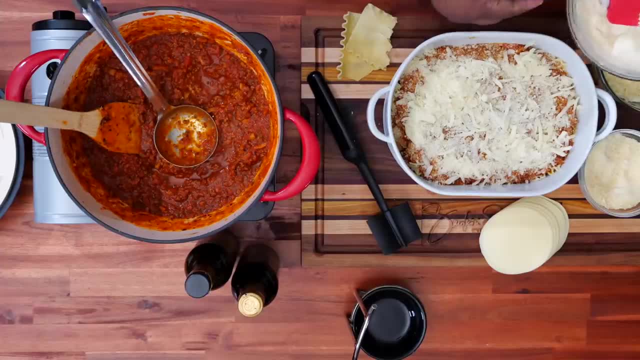 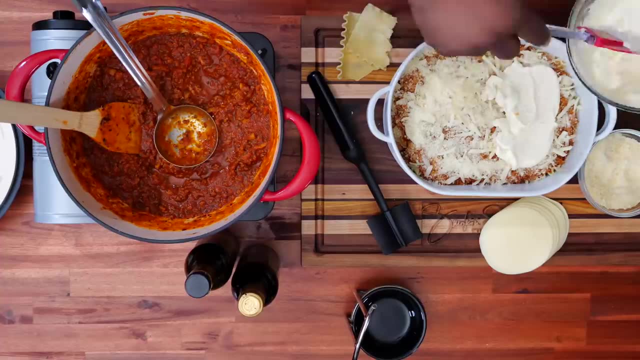 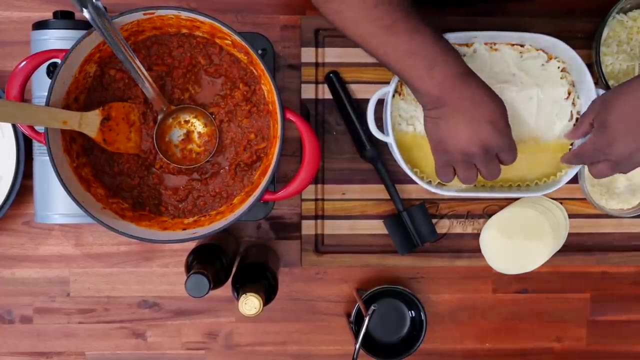 whirl, just like. you see, we just want to add a nice little layer to here too. i'm not going to bore you guys, but we're going to do the same thing we did down at the bottom right. and again, folks, i'm doing it a little bit of a hard way only because i wanted to use my nice 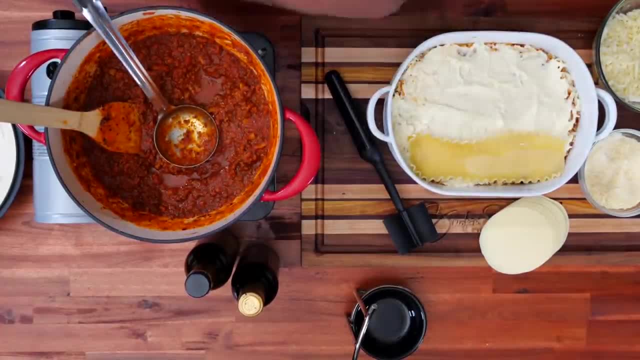 this is my good looking dish right here. so i'm going to put a layer of noodles, then we're going to go with some meat sauce, and then we're just going to go with the cheese, and we're just going to keep doing that until we get to the top. 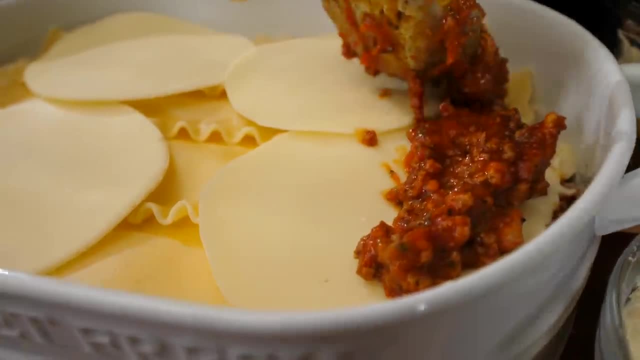 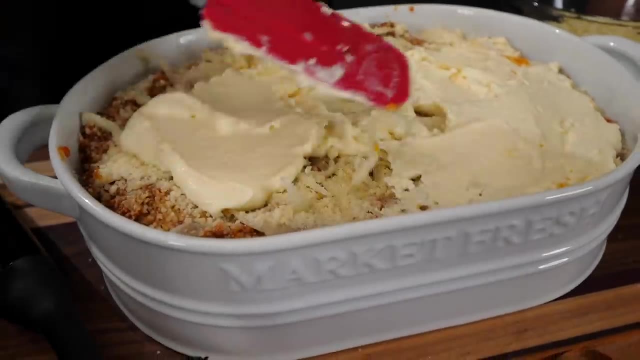 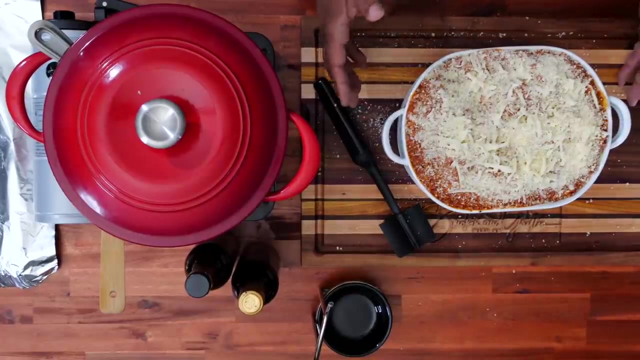 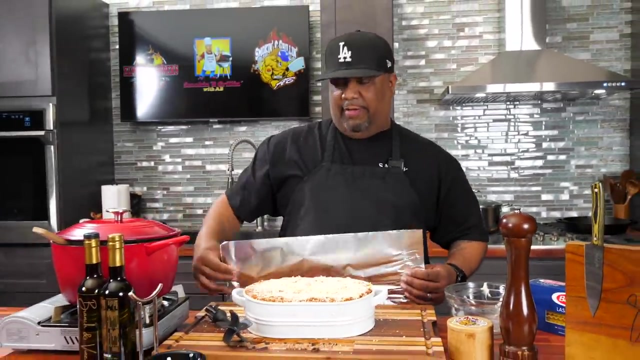 so, as you can see, look, i got it all the way up here to the top right. this is kind of like a lot, you know what i mean? 13 by 9 would have been better, especially because we know we got to put foil over the top and i don't want to pull none of my cheese off, right? so, look, i got a. 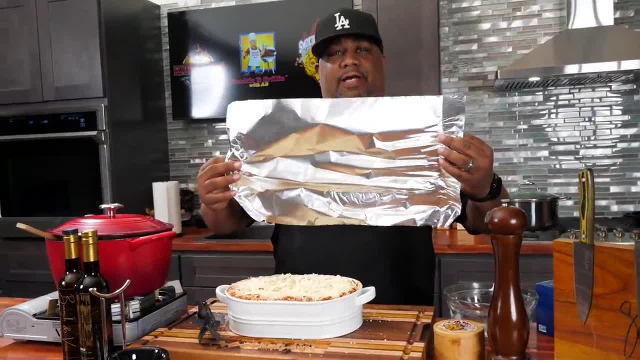 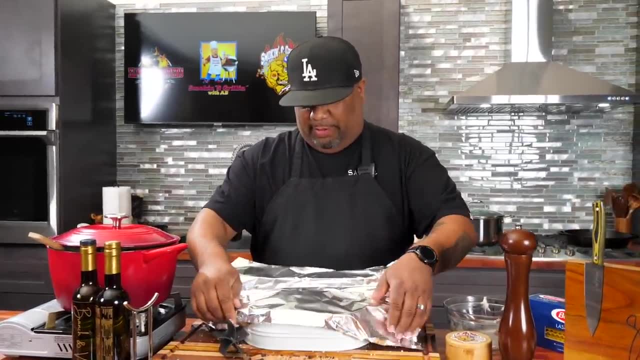 question for y'all: tell me, you see the floor this side, this side, how many of y'all know know which way the foil is supposed to be? let me know down in the comment section below. so look, i'm gonna just put it over here like this and i'm not gonna like make it go. you know i don't want it. 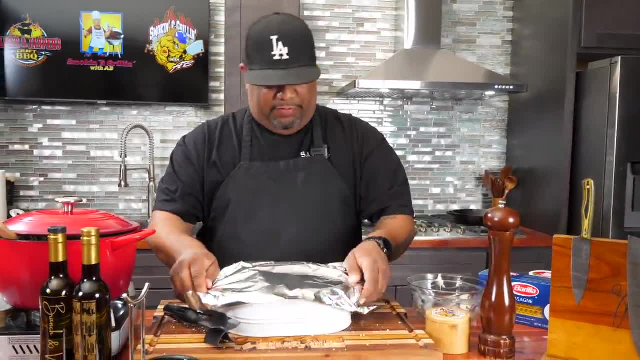 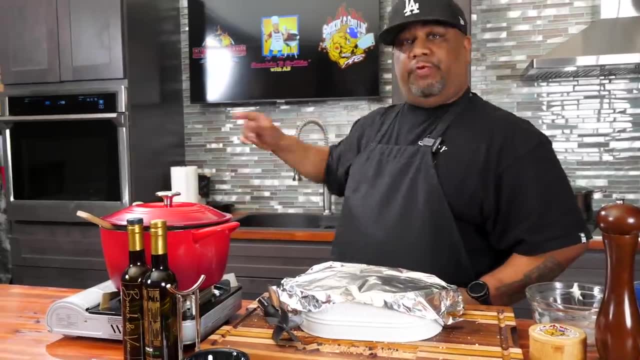 to just like actually touch my cheese. what i'm gonna do is i'm just gonna cover it this way and, because of my dish is so full, what i'm gonna do is- which i've already done- is i already preheated my oven to 375 degrees. we're gonna let that stay in there for about 40 minutes, but i put a pan. 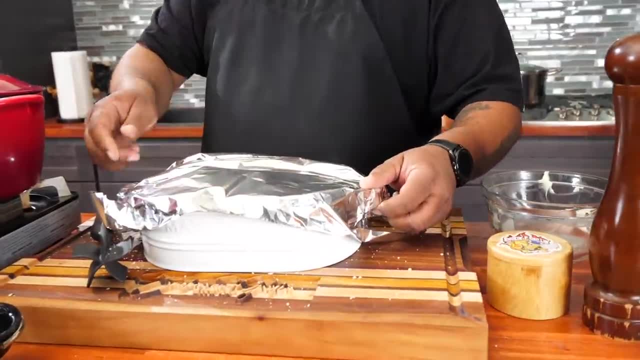 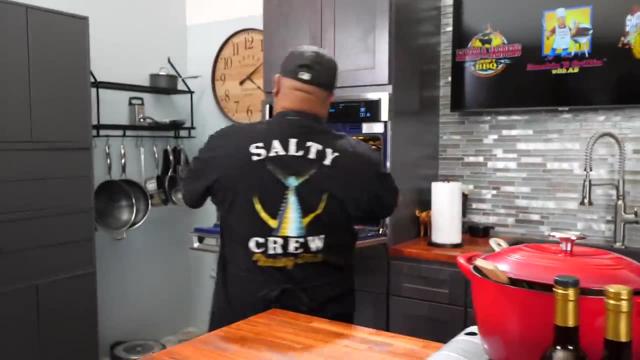 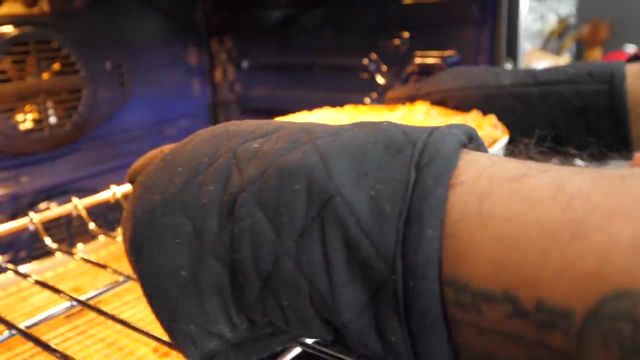 underneath the bottom. that way, you know what? because i clean up my own this way. when i put this in there, anything that bubbles over the top drops down in that pan. a little pro tip folks. okay, there it is. folks. y'all tell me what you think about that there. that right, there is going. 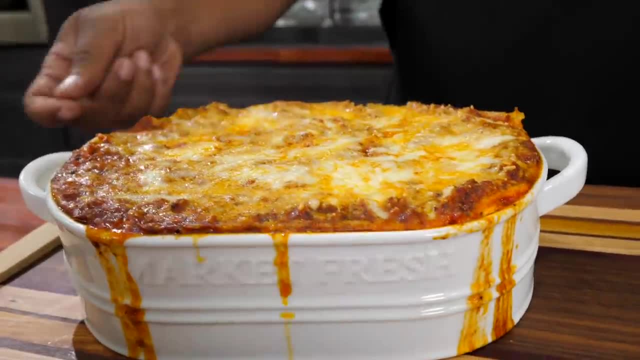 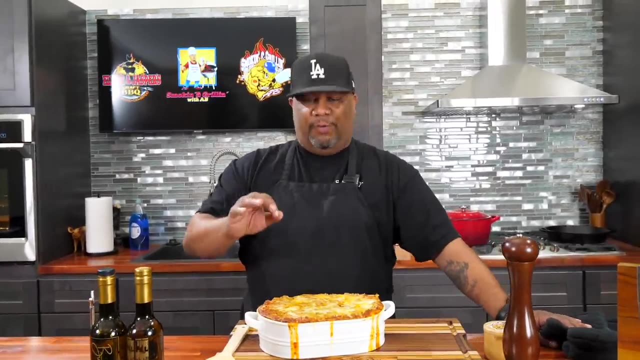 to be fire. look, so after 40 minutes you take the foil off and then you go back in for about 10 minutes because what you want to do is you want to like melt that and get a little crust on the top right, super easy. hey, overly delicious all of that, and you know why i know it's delicious. 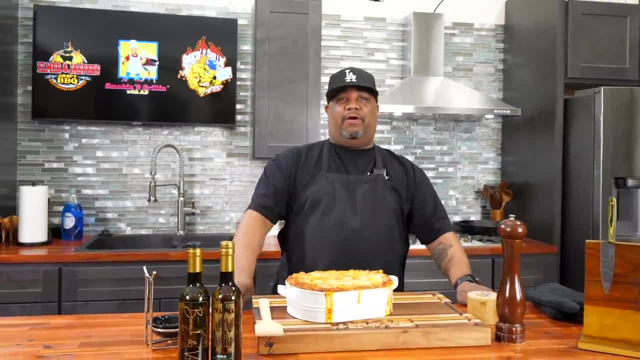 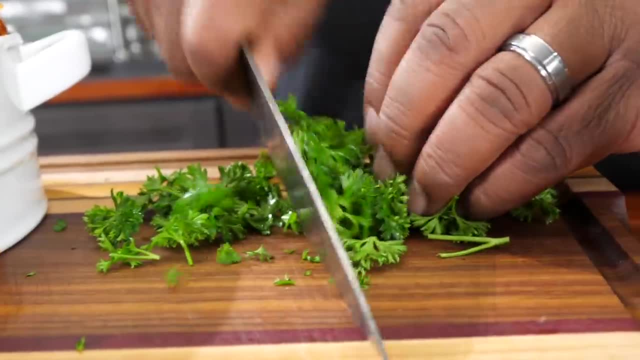 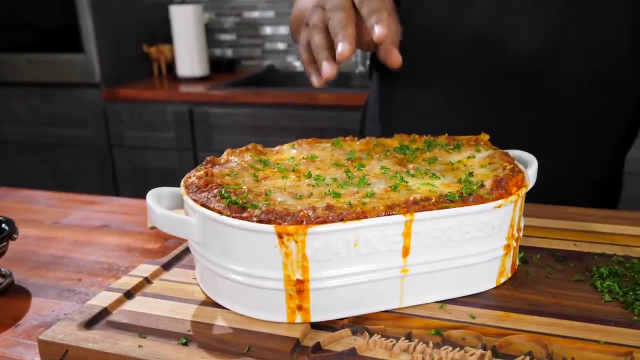 because, check this out, i don't even have to do that. oh man, this is going to be incredible, hey. so what we're going to do is we're going to let this rest for about 15 minutes, and then we're going to cut into it, plate it, and then we're going to eat it. hit it with the, you know the. 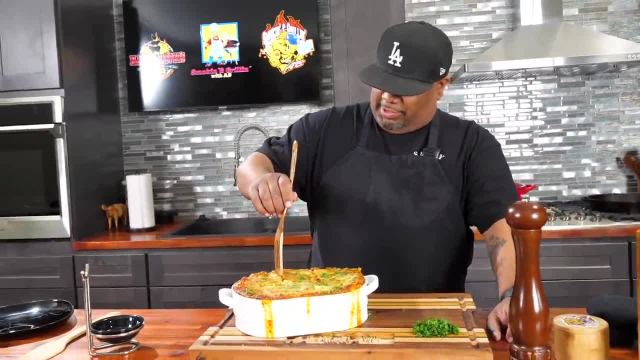 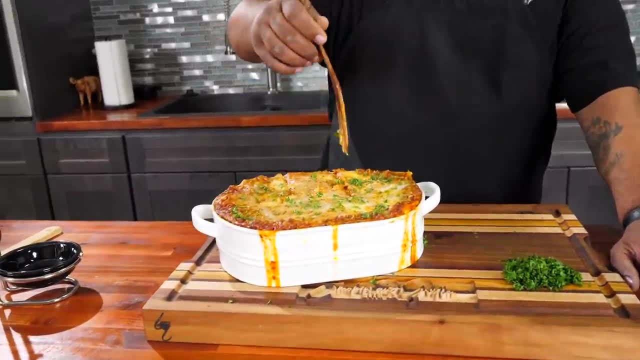 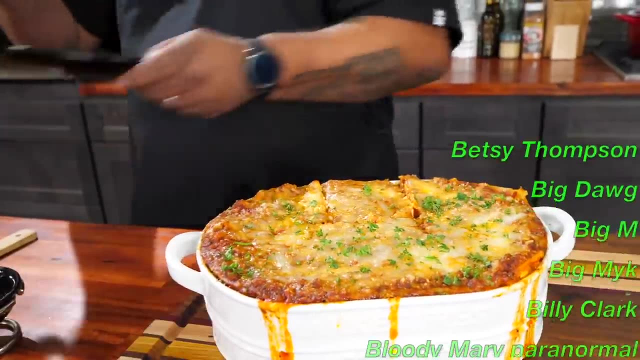 i guess we call them the money shots, right? so now i'm gonna go ahead and just cut this here. oh my goodness, you see that. oh, y'all probably didn't even see that, but when i pull this up, look at that a little bit of that cheese pull. oh yeah, this is where it gets tricky folks. so now i'm 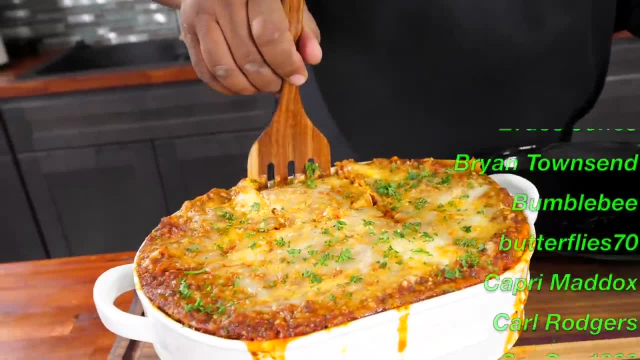 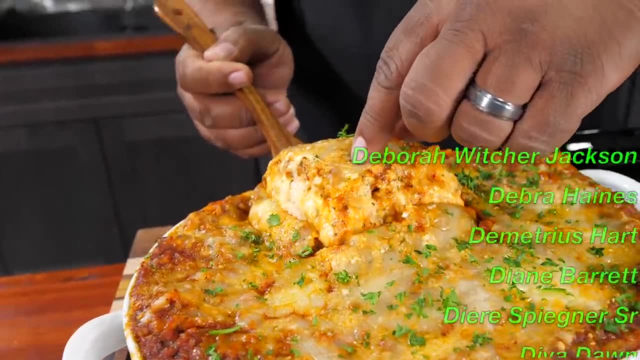 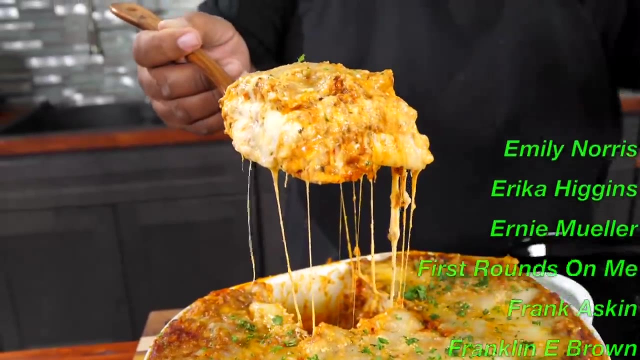 gonna take this now, we're gonna go down this way and we're gonna attempt, attempt to get underneath it. pull it up right here, pull it up and see if we can't get that out like that. ah, my goodness folks. so once that's cut, the other established. so i won't look any stronger like i did the other. 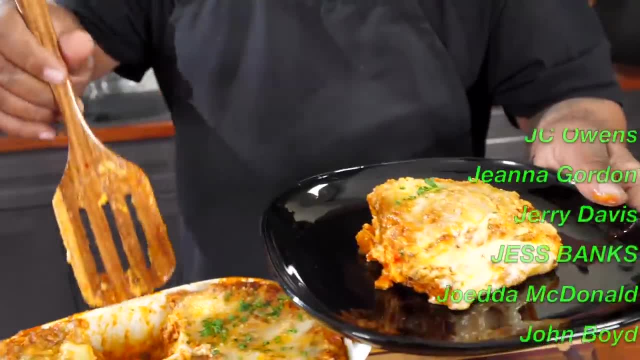 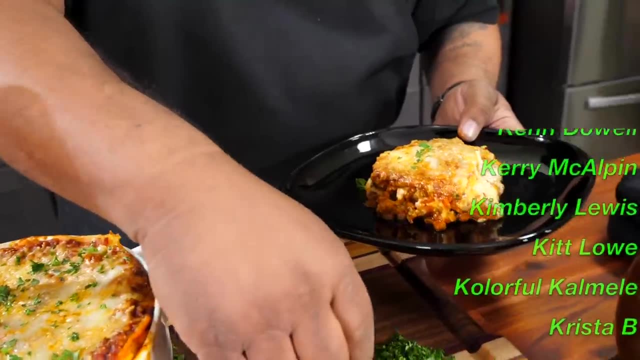 hand, let me go ahead and do that, and that there is what i'm gonna call a piece of lasagna. look at that, and therefore all my people that's really into that. uh, that presentation, let's just go ahead and get us a little bit, a little bit more. 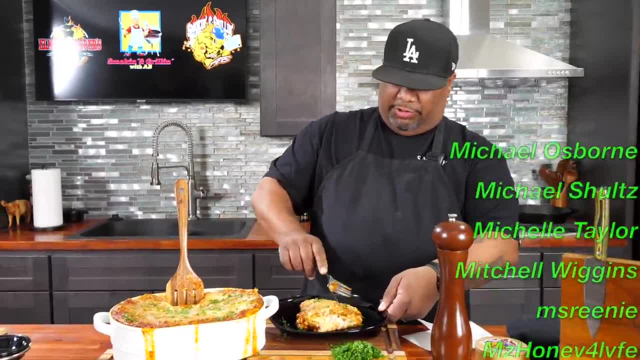 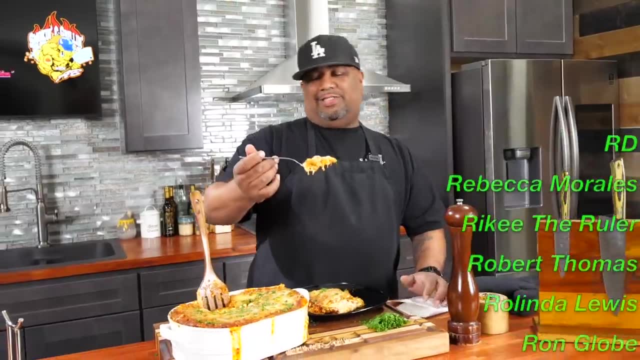 garnish. okay, folks. so look, now it's time to just to get on in. i told you guys when i first started, But I can tell you, the ricotta, all the cheeses, I mean this is just deliciousness on a fork. Now, don't forget, we let it cool for about 15 minutes, right? 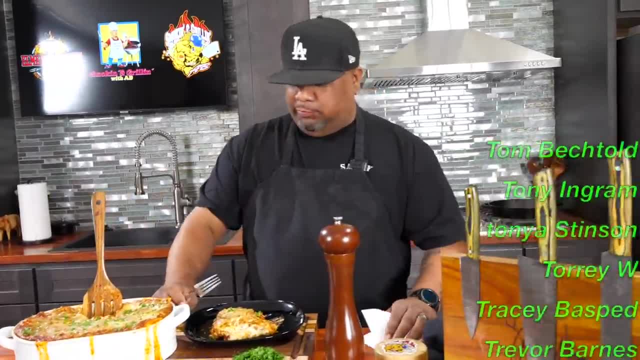 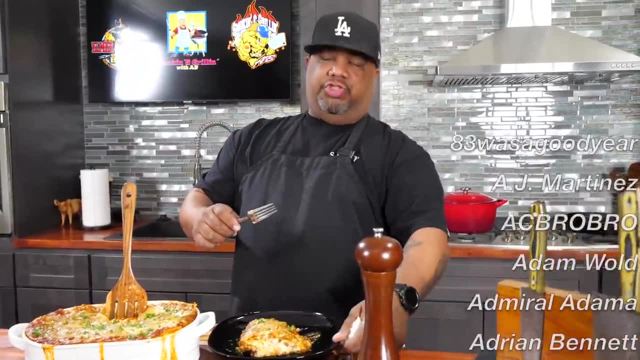 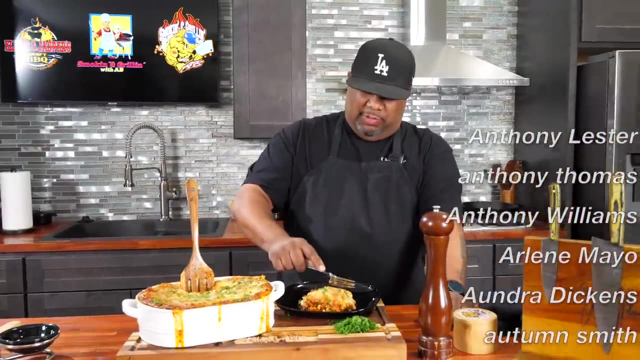 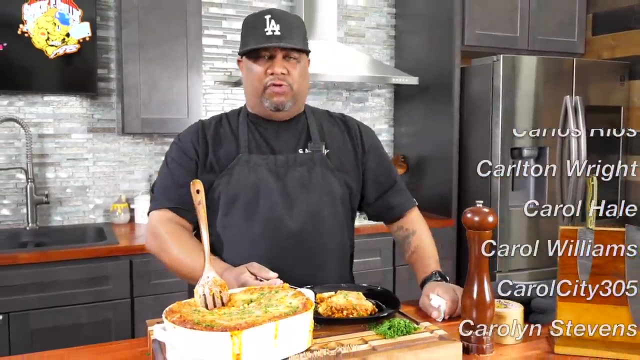 Mmm, Mmm. Now I don't know, The jury's still out. They got you know. it's like a deadlock, meaning we got to go back and taste it again. But I can tell you this right now: the bite you know, and that spiciness from that red you know, chili flakes I can, oh man, that's just perfect. 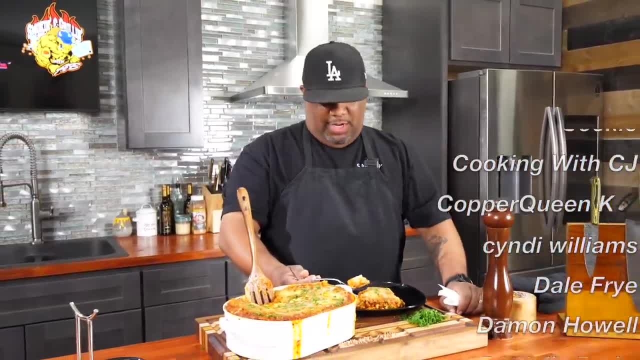 But for all you guys that like to have it a little bit hotter, you can go ahead and I can say it'll take a double and just about anybody can eat it Right now. it's just like playing, it's like a hint on your palate. 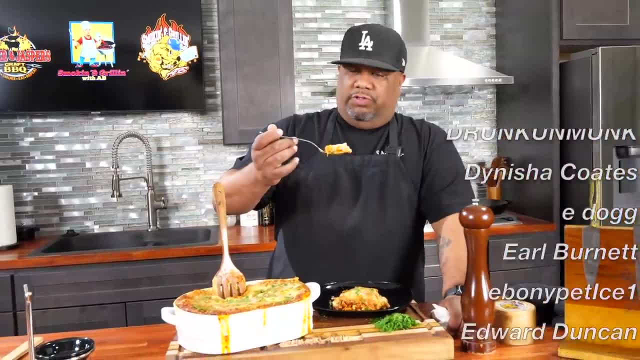 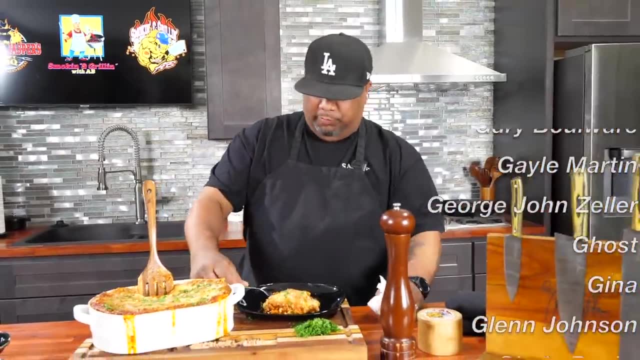 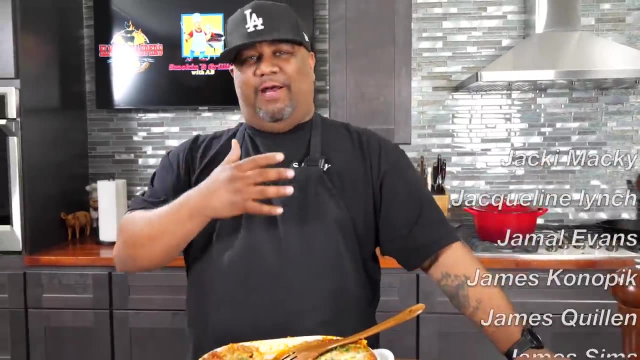 Mmm, Real nice. And the meat for those of you guys that eat pork. you know that beef and pork combination that does it too. Mmm, Hey, I was just supposed to take a couple bites, wipe my mouth and then tell you guys. you know what I thought about this, right.